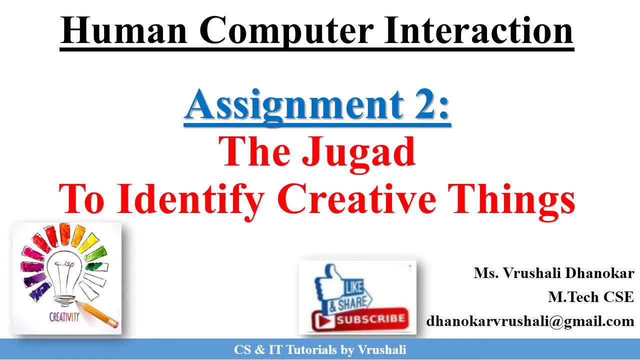 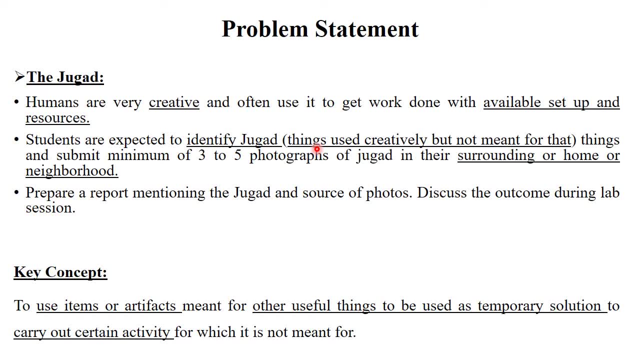 You need to identify the creative things in your surrounding. This is your second assignment, So let's see The problem statement of your second assignment is the Jugaad. Here, humans are very creative and often used to get a work done with available setup and resources. 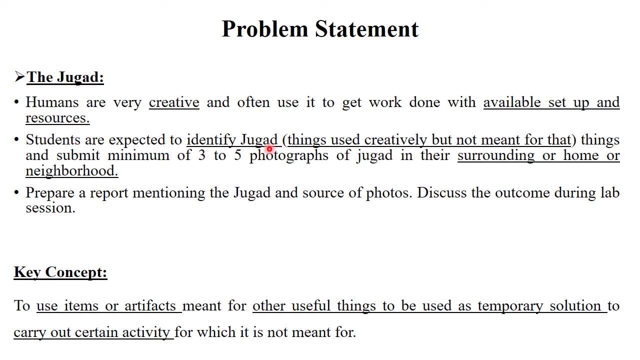 right. So in this assignment, students are expected to identify Jugaad. Jugaad means things used creatively but not meant for that, Okay. so you need to identify those types of things And submit minimum of three to five photographs of Jugaad in their surrounding or home or 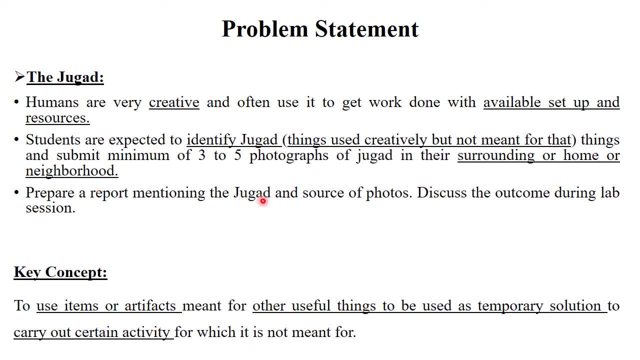 neighborhood And you need to prepare a report mentioning the Jugaad and source of photos and discuss the outcome during the lab session. So this is a problem statement or this is an assignment that I have mentioned in your syllabus. So the basic, key concept behind 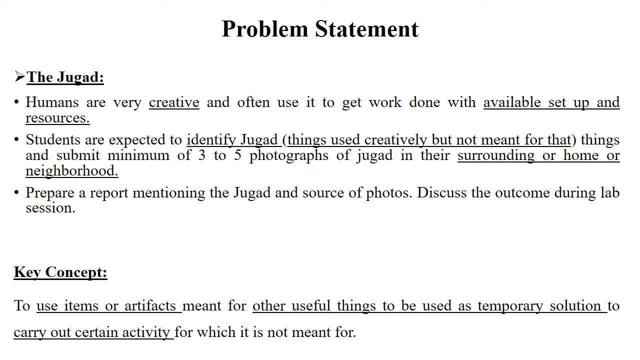 the Jugaad is you need to use different items, different waste materials or artifacts. By using those items, you need to make a proper activities or you need to make a proper product. Okay, So this thing is called Jugaad means by using a particular thing, you need to provide a different solution. 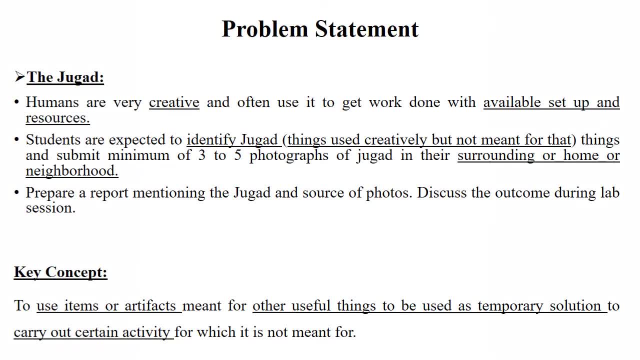 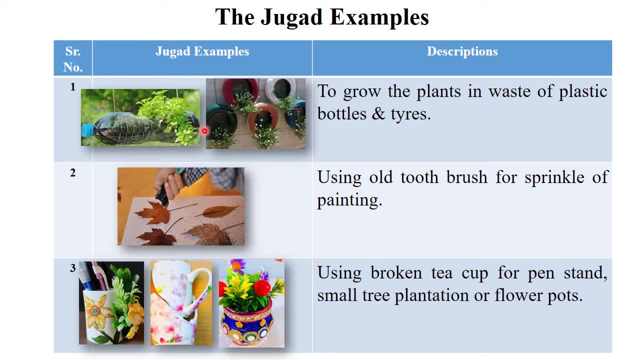 right. So let's see the example of these things Now. just see here. the first example is plastic bottles. We know that the plastic bottles like oral bottles and other plastic wares. this is a very difficult things, Right, and this is a system where 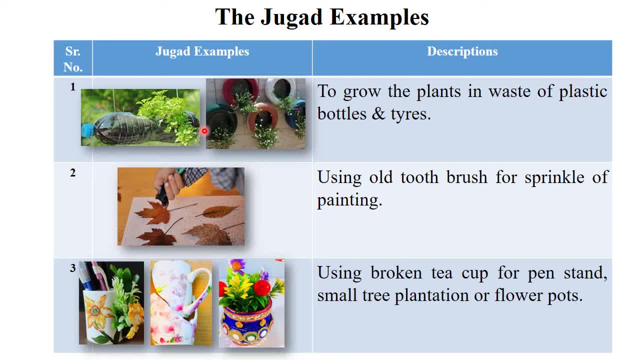 you can use time, use space, not a decomposable right- so you can use those plates, plastic bottles or tires to grow the plants. so this is the best jugaad examples regarding the plastic wares, or by using the tires, so that will be useful to growing the plants. now, next one is old toothbrush. you can use old toothbrush for 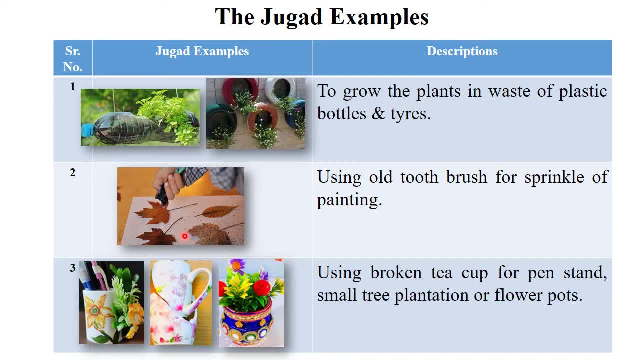 sprinkles of painting, if anyone student or anyone having the interest in drawing or painting, so you can use the old toothbrush for sprinkling purpose right now. the next one is in your kitchen. there was sometimes a broken tea cup right or broken cups having there, so you can use those broken cups. 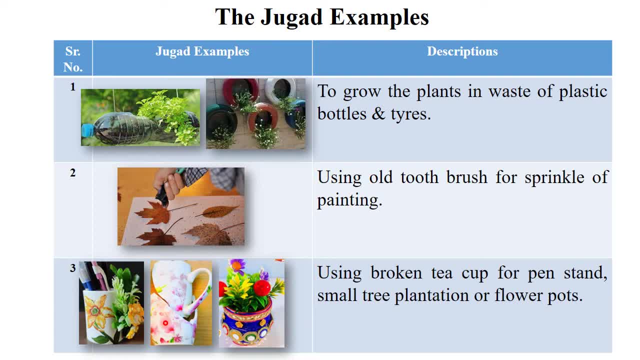 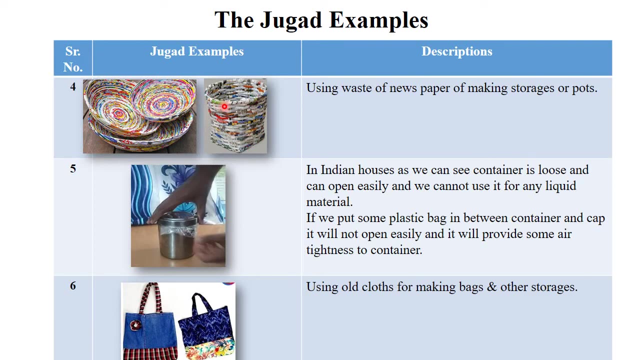 creatively. you need to use different craft ideas and use those broken tea cup for paint stand or small tree plantation or like flower pots. so this is also one kind of jugaad examples. next, the next one is a newspaper in your home, delhi newspaper, having there right, so you can use those newspaper for making a creative. 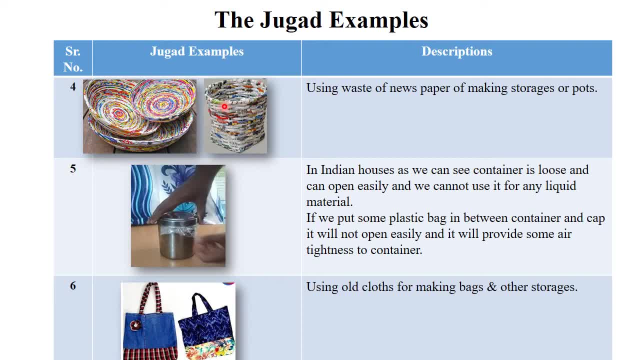 things. okay, anyone having the interest to make a creative things or, in particular, craft side or craft domain, so you can use the newspaper for making a particular storages or making a particular pots right now. the next one is: see, i think you all are familiar with this example- in indian houses we 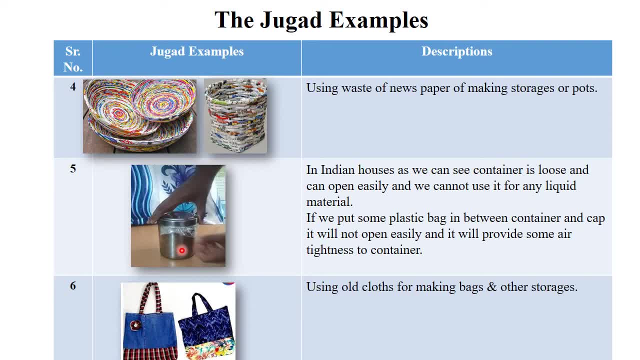 can use the newspaper for making things right. but sometimes this kind of containers or steel containers having a very loose and can that they can open easily, right, we cannot use any liquid material in this particular container or box, right? so what we can do, we can put some plastic bag in. 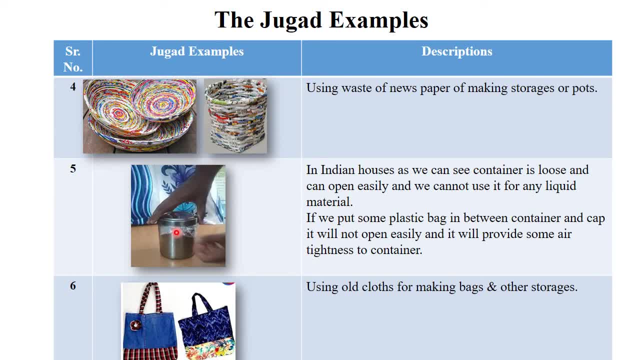 between those container. okay, so after putting plastic bag, this cap it will not open easily, right? because this particular plastic bag provide some air tightness to this particular container, right? so this is also one kind of jugaad. means you can also carry liquid material through this container after putting this plastic bag. means this container make a air tightness. 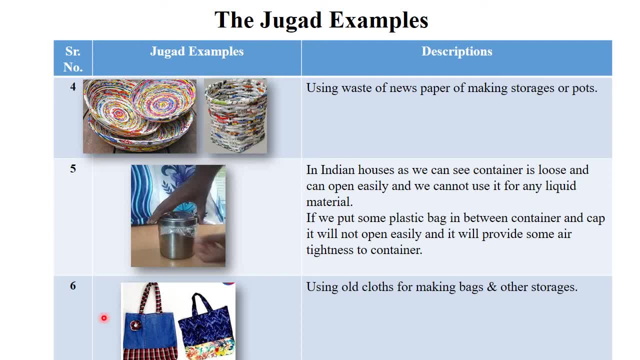 having there right now. the next one is old clothes. you can use old clothes for making a bags and other storages. there are different shops having there. they can use this old clothes and they can provide the particular particular bags or storage stock in it particular particular storage area by using this old clothes. so you can use those thing. 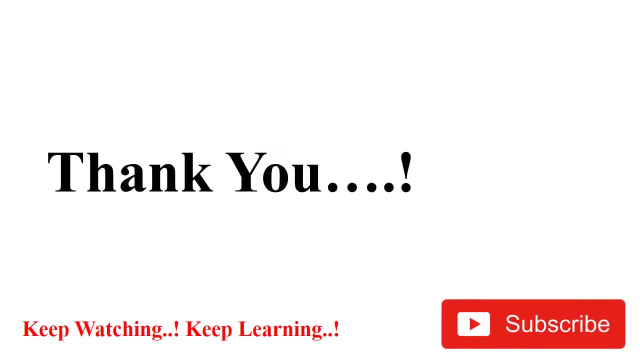 so these are the some jugaad examples. so these are the some jugaad examples. you need to also search different jugaad examples in your surrounding and mention in comments. so you need to make a proper report regarding this particular assignment. okay, so all the best, thank you.